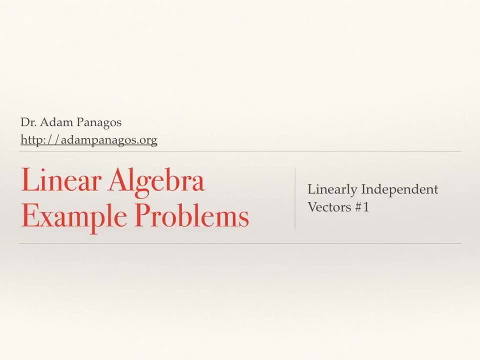 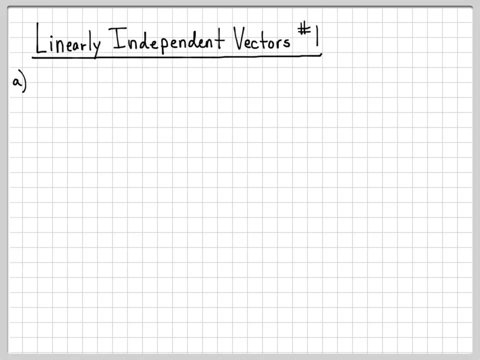 We're going to look at a set of vectors and determine if they are linearly independent or not. So we'll do this two different times In this first part. we're going to look at the vectors 2, 2, 1, and negative, 4, 6, 5, and 1, 0, 0.. And we're asking the question. 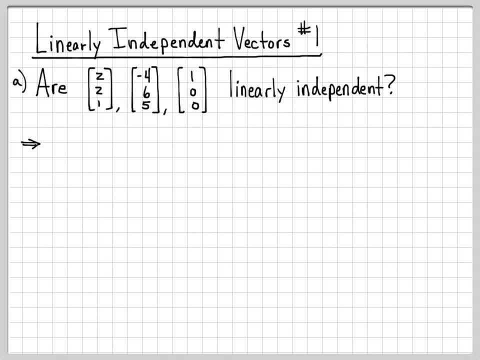 are these vectors, this set of three vectors, linearly independent? So recall what it means for vectors to be linearly independent If this linear combination of them. so if I take a number alpha 1 times the first vector, a number alpha 2 times the second one, and a 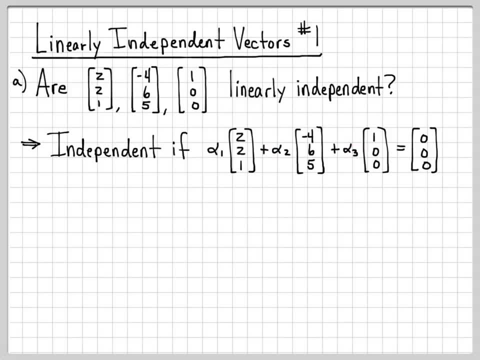 number alpha 3 times the third one, if this linear combination is equal to the all 0 vector, if this has a solution that is only the trivial solution, meaning if the only way that I can find alpha 1,, alpha 2, and alpha 3 to force this linear combination to be all 0s, if the 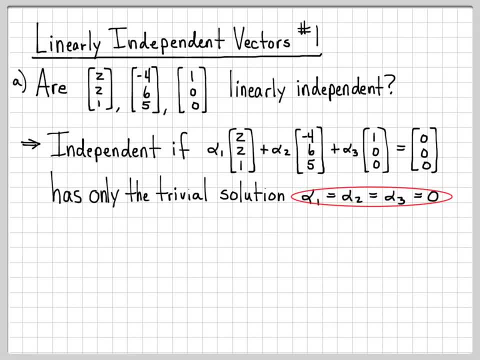 only solution to that is alpha 1,, alpha 2, and alpha 3, if the only solution to that is the trivial solution, when alpha 1,, alpha 2, and alpha 3 are equal to 0, then we say: 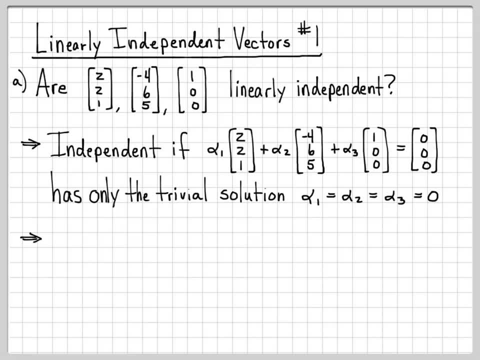 that the vectors are linearly independent. If there's another solution, if I can find alpha 1, alpha 2, and alpha 3 that yield the all 0 vector, such that alpha 1, alpha 2, and alpha 3 aren't all 0, then we have a non-trivial solution and we say that the vectors are. 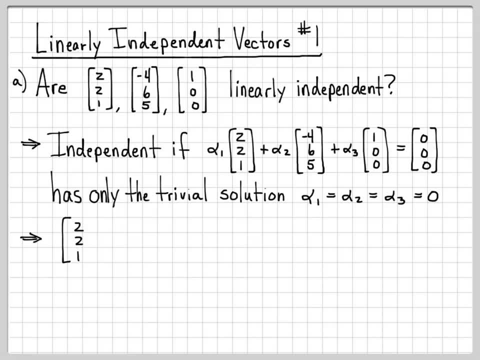 dependent. So how can we figure this out? Well, we can do this by constructing an augmented matrix and figuring out if we can solve for the coefficient of alpha 1,, alpha 2, and alpha 3.. If it turns out there's only the trivial solution, then we say they're independent. 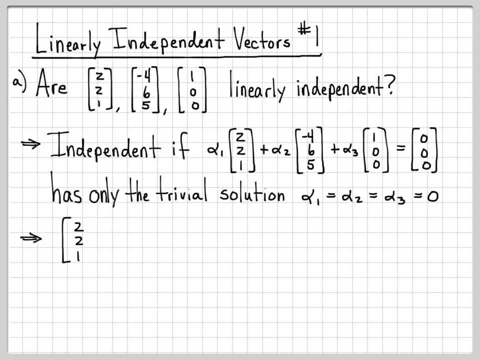 If there's more than the trivial solution, then we say they're dependent. So let's go ahead and form the augmented matrix. The first column is the first vector, the second column is the second vector, the third column is the third vector and then the fourth column. 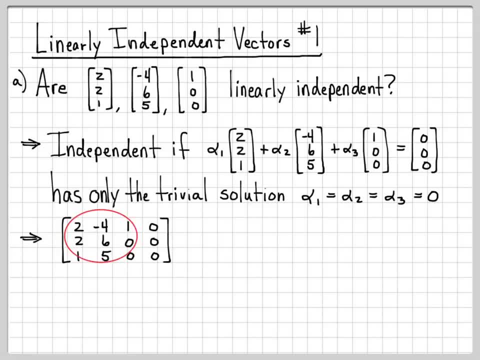 is the all 0 vector, because that's what we're seeing. if we can find a solution for I call this the augmented matrix, as usual. So that's our augmented matrix, And then we're going to go ahead and form the matrix And then, if I perform row reduction and we're not, 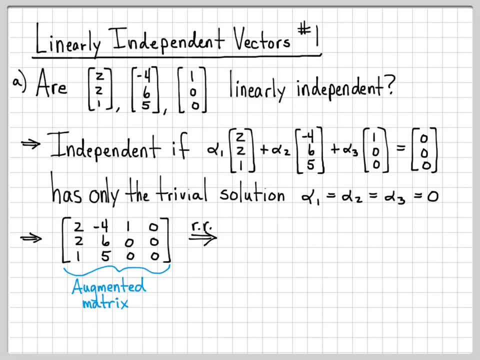 going to do all those steps here. I have lots of other videos where we go through those details of how you do that exactly, But if I perform row reduction steps, I'll end up with a row-reduced matrix that looks like this: So when I look at this, we have a pivot 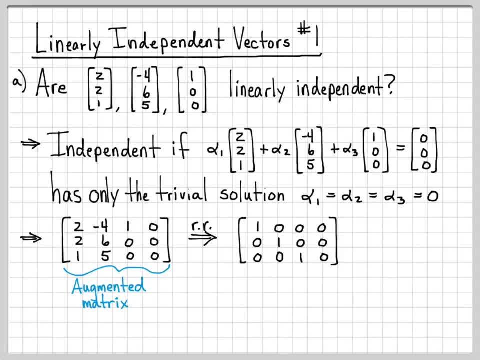 in every single column. So there are no free variables, There are just three basic variables: alpha 1, alpha 2, and alpha 3.. And when I look at this, if I look at the first row, this equation right here says that 1 times alpha 1 plus 0 times alpha 2 plus 0 times alpha 3 equals 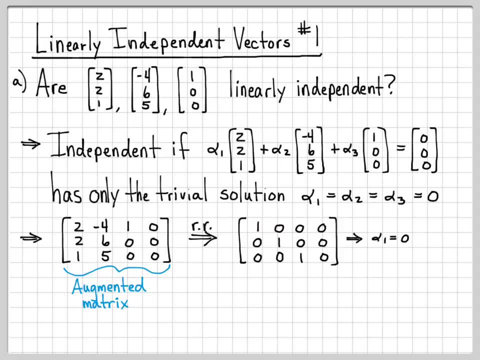 0,, which means that alpha 1 is 0.. Similarly, when I look at the second row, this line here tells me that alpha 2 is equal to 0.. And the third line tells me that alpha 3 is equal to 0.. So the only solution to this system of equations that I've constructed is the. 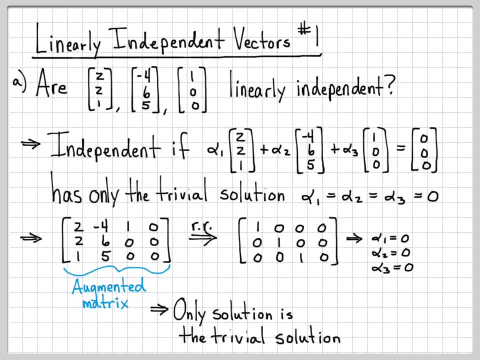 trivial solution. So the only solution is the trivial solution, And that means that these vectors are indeed independent. So we have determined that these vectors are linearly independent vectors. Let's do another example. So same: first, two vectors, but the third vector. 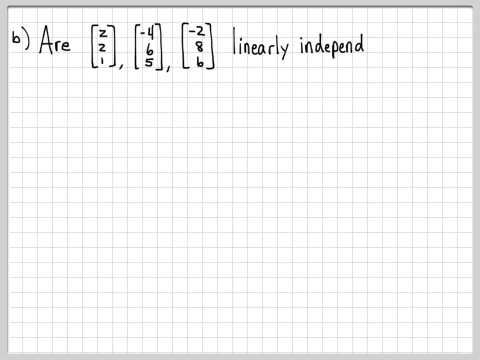 I'm going to change to be negative. 2,, 8, and 6.. Are these linearly independent? Again, we know how to check this. If the linear combination of these vectors, equaling the 0 vector, has only a trivial solution, then they are linearly independent. 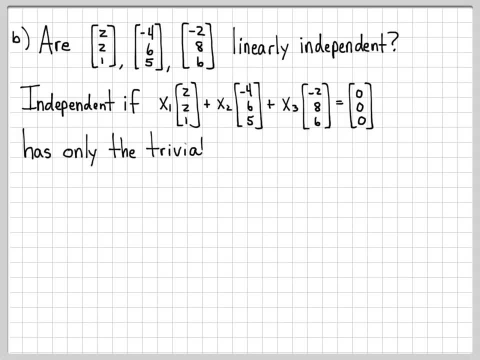 If there is a nontrivial solution to this equation, then we know they are dependent. So that's our statement. again, How am I going to figure this out? I'm going to form an augmented matrix: Column 1,, column 2,, column 3.. And they all 0 vector. I need to solve this system. 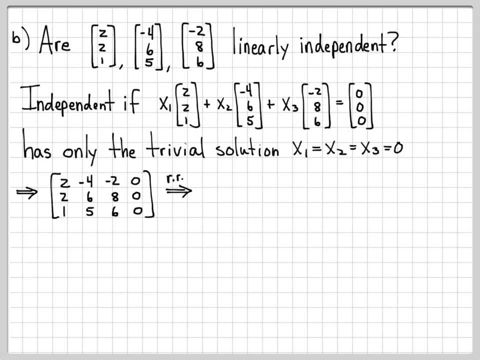 of equations. If I perform row reduction, this turns into the matrix that looks like this: This looks a little bit different than the first time because we've changed that third vector. It's going to have a different solution. I have a pivot. If I had a pivot. 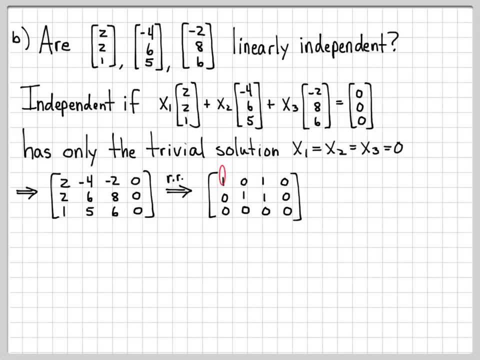 this would have been negative. But if you had a pivot it would have been negative. I can. I have a pivot in the first column. here's a pivot. I have a pivot in the second column. So we know that x1 and x2 are basic variables. that leaves x3 as a free variable. So x1 and